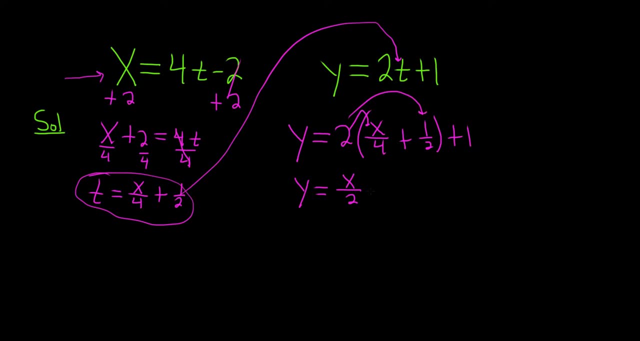 And then 2 times 1 half is well, it's just 1, so plus 1.. And then we still have this other 1 over here outside the parenthesis. So if y equals, let's write it like this: 1 half x plus 2.. 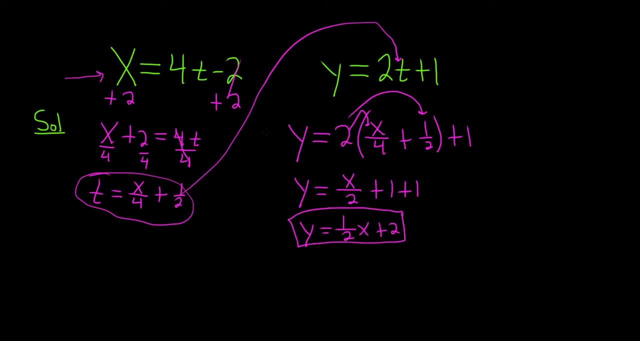 So this would be the rectangular equation. So these are the parametric equations and this is the rectangular equation. All right, this is just a line, right, mx plus b. Let's do a quick graph. So here's the y axis. 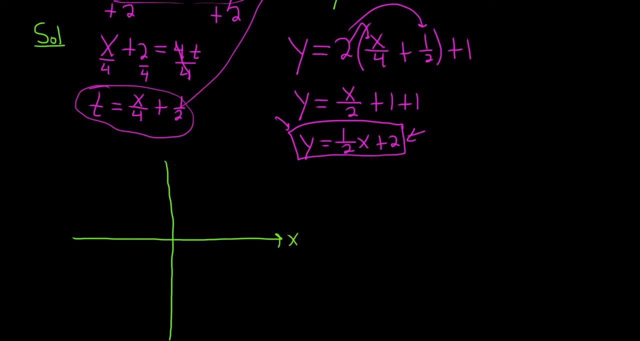 Here's the x axis And let's see: 1, x is 0,, y is up here at 2.. Let's put a dot And I guess if you were to set this equal to 0, you could find the other intercept. 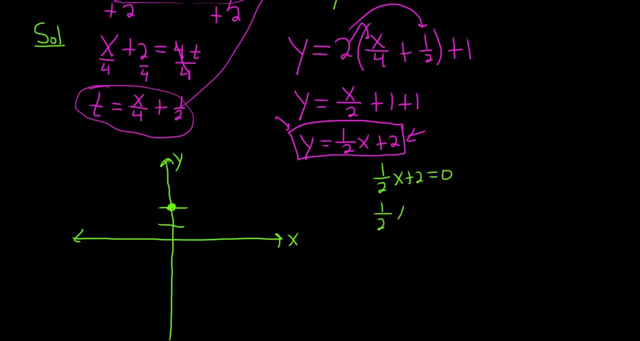 It's not necessary, but why not? So 1 half x is negative 2. We'll multiply it by 2. You get x equals negative 4.. Yep, so over here. 1,, 2,, 3,, 4,. we have another dot. 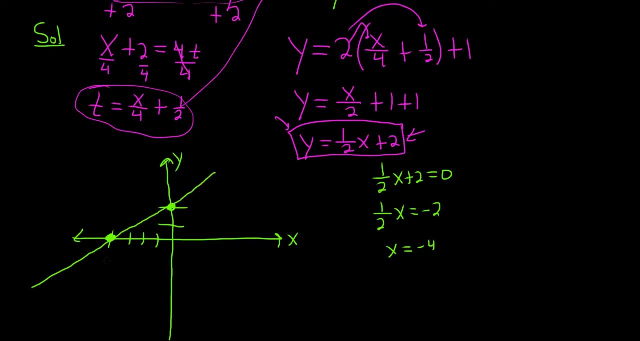 So it looks something like this: Notice, I have not put arrows on the end of my line, because now we're going to indicate something called the orientation. So, to find the orientation, what you do is you make a table, So t and then x, and then y, And I don't have it on the screen. 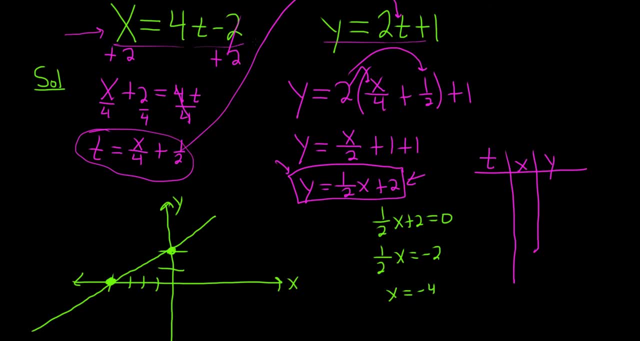 so I'm going to scroll up a little bit so we see it. Okay. So there's our x up here: 4t minus 2, and our y is 2t plus 1.. Then you plot points in increasing values of t. 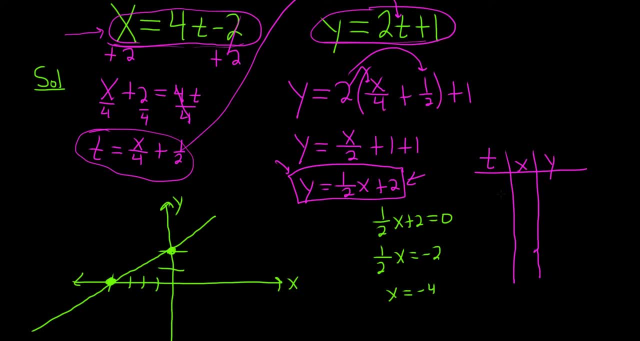 and that will indicate the orientation on the graph, Again in increasing values. So let's try like 0, and let's try, you know, 1.. That should be good enough. So plugging in t equals 0 into our first equation for x. 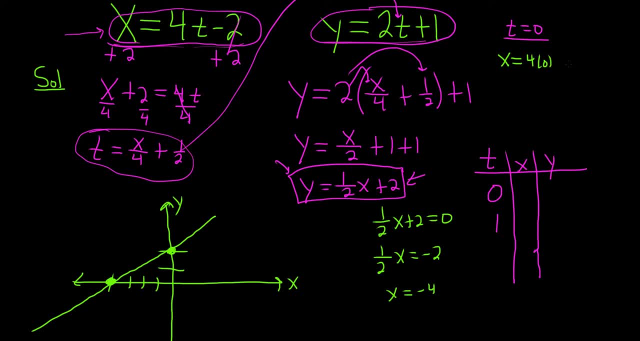 we'll get 4 times 0 minus 2.. So 0 minus 2,, so minus 2.. So I'm going to come over here and then just fill in the table And then y, that'll be 2 times 0 plus 1.. 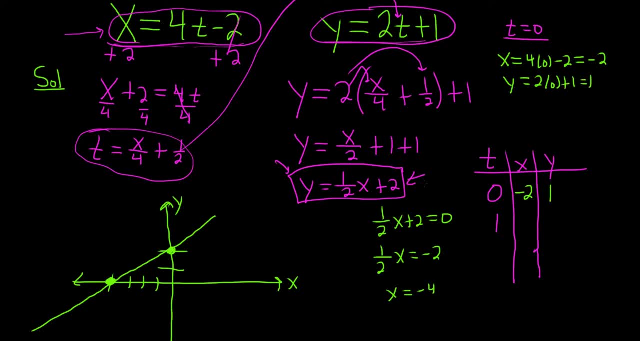 So 0 plus 1,, so 1.. So we're here. So when t is equal to 0, we are right. I'm going to use a different color so you can see it. We're at negative 2 comma 1, which actually our line was a pretty good line. 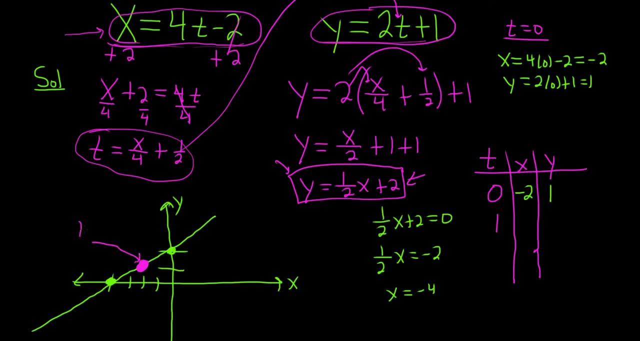 So there is the point. It is the point on the graph that corresponds to the value of the parameter. t equals 0.. Now let's do t equals 1.. And again, we could have picked any number you know bigger, and that would have been fine. 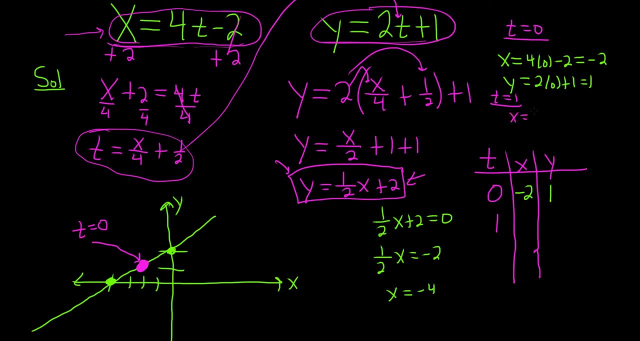 Okay, So we'll have x equals 4 times 1 minus 2.. So that's just 2.. So I'm going to come over here and fill it in, And then y equals 2 times 1 plus 1, so 3.. 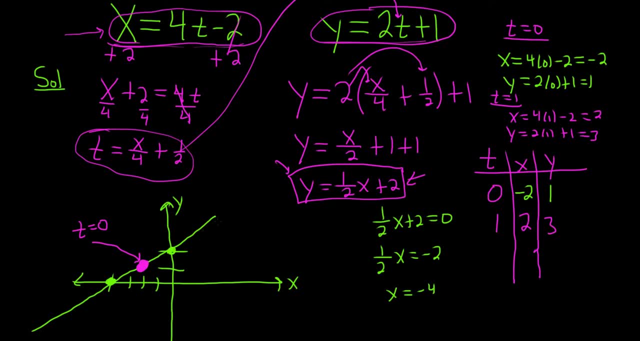 So 3.. So when t equals 1, we're at the point 2 comma 3.. So 1, 2.. So 2 comma 3.. So maybe it's right here. So this is the ordered pair on the graph that corresponds to t equals 1.. 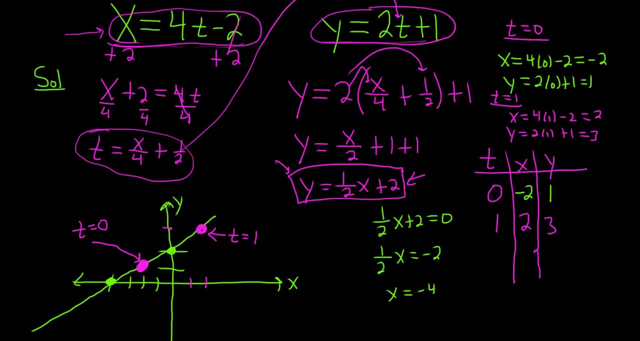 So you see, as time passes, the parametric equations give you points on the graph And you can use parametric equations to describe any type of path in math. So you see that we're going from 0 to 1.. So it's going this way. 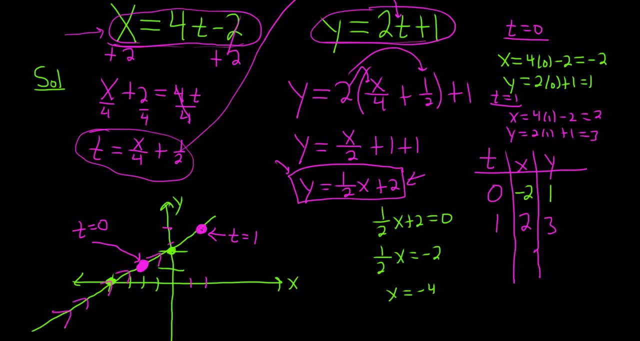 So you indicate that by drawing several arrows. So this would be a perfect graph, right? We have the graph of the parametric equations and we have indicated the orientation, And again this one is called the rectangular equation. I hope this video has been helpful.